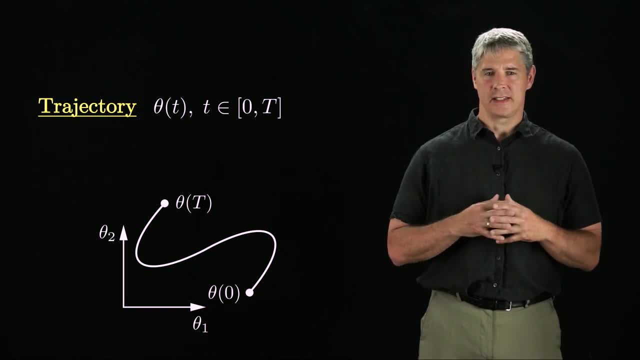 follows the path shown here. In some cases, it is desirable to separate the C space path from the speed at which it's followed. For example, we might plan a geometric path for a mobile robot to avoid obstacles on the floor without worrying about how fast the path is followed. 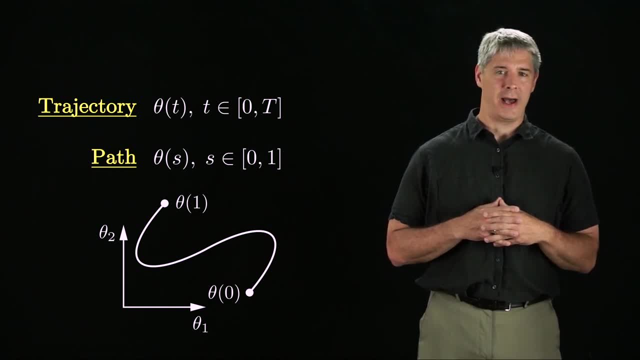 We define a path to be a curve in configuration space as a function of a path parameter s that goes from zero to one. As s increases from zero, the robot moves from the start- configuration at theta of zero- to the end configuration at theta of one. A path can: 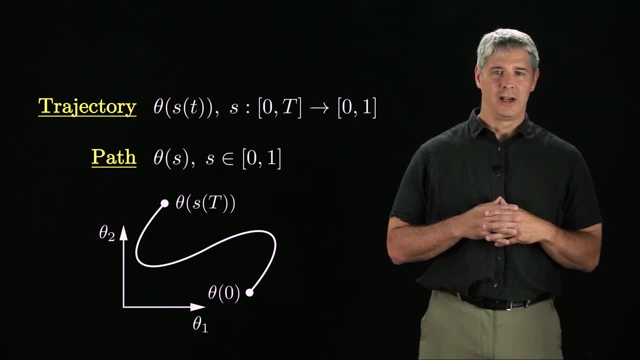 be turned into a trajectory by defining a function s of t which maps the time range zero to capital T to the path parameter range zero to one. This function is called a time scaling. The time scaling controls how fast the path is followed. Now, with the trajectory, theta of s of t, the time derivative of theta dot is: 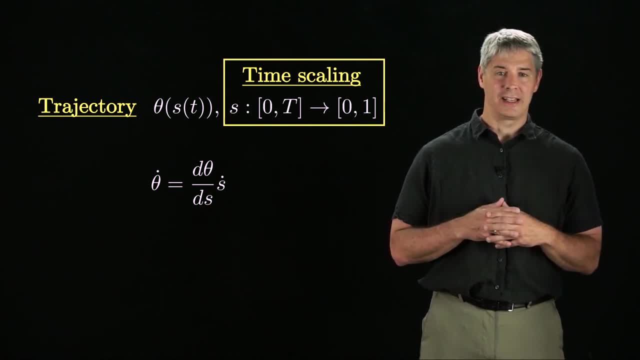 determined by the chain rule to be d theta d s times s dot. The acceleration theta double dot is determined by the product rule and the chain rule to be d theta d s times s double dot plus d squared theta d s squared times s dot squared. Since the dynamics depend on 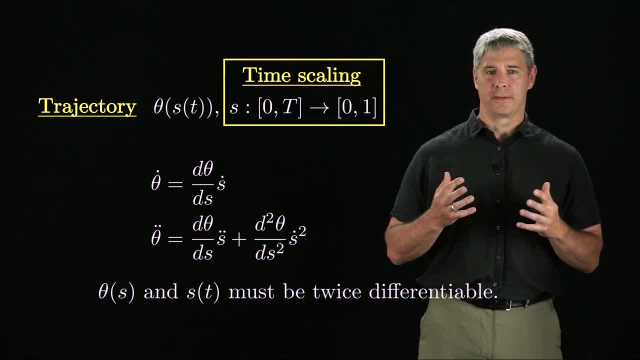 theta double dot. for the dynamics to be well defined, the second derivatives of both theta of s and s of t must exist. In this chapter we consider the problem of planning paths and trajectories without considering obstacles. In chapter 10, on motion planning, we address the case of obstacles in the environment. 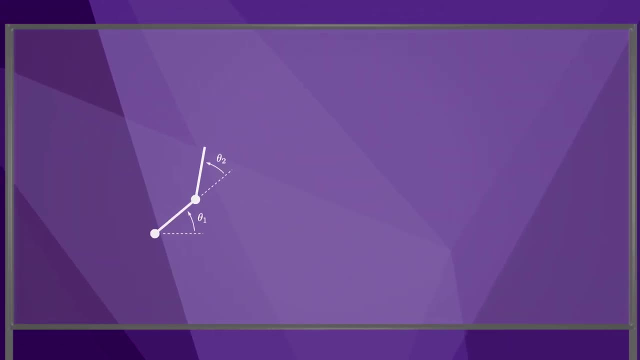 Let's start by planning a path for a robot arm in its C space. The simplest type of path is a straight line path from an initial configuration, theta start, to a final configuration, theta end, As described by this equation: As s goes from 0 to 1, the configuration goes from theta start. 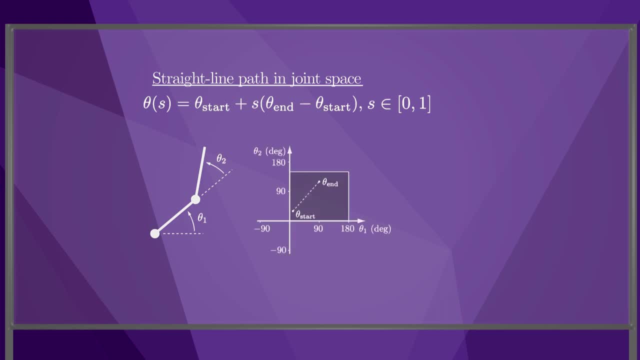 to theta end. A straight line path in joint space is shown here for a 2R robot with 180 degrees of motion about its first joint and 150 degrees of motion about its second joint. The path can also be visualized in the work space as shown here. Note that the end point 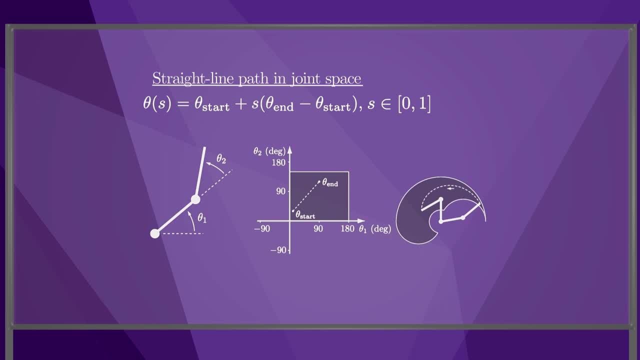 of the robot does not follow a straight line. If we prefer a straight line motion of the end effector in Cartesian space, we can define x to be the coordinates of the end effector and define a straight line path, as shown here. Then we have to use inverse kinematics to solve for the robot configuration. 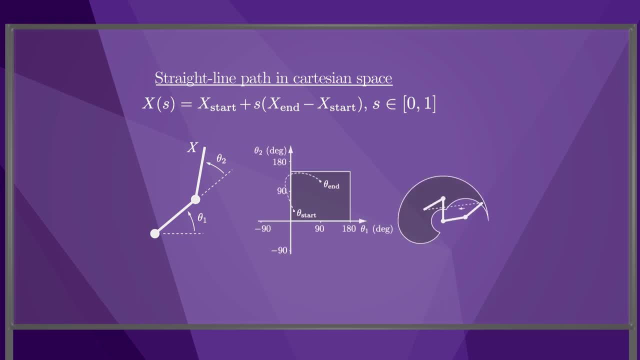 at each point along the path. As you can see here, some straight lines in Cartesian space cannot be executed as they pass outside the work space. One advantage of planning straight line motions in joint space is that the joint limits are usually independent of each other, so the set of feasible 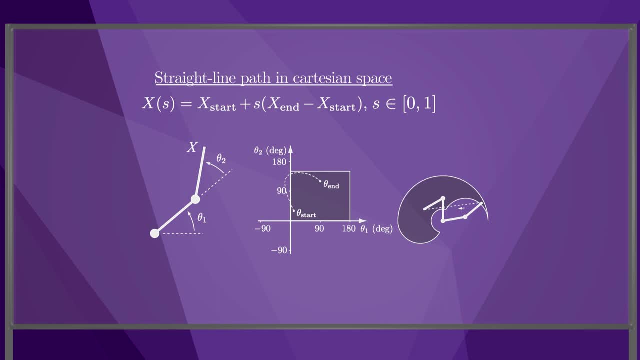 joint configurations is convex. unlike the work space. A straight line between two points in a convex space always remains inside the space. We can also plan a path between two rigid body frames represented in SE3.. We could try directly extending our straight line definition in joint space, but of course this does not. 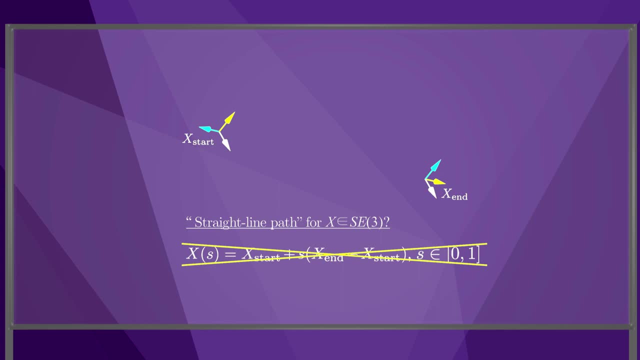 make sense. There is no meaning to subtracting two elements of SE3.. Let's find the screw path where the frame follows a constant twist from x start to x end. First let's express the frame x end relative to x start. Each of X start and X end is implicitly defined in a space frame S, so by our 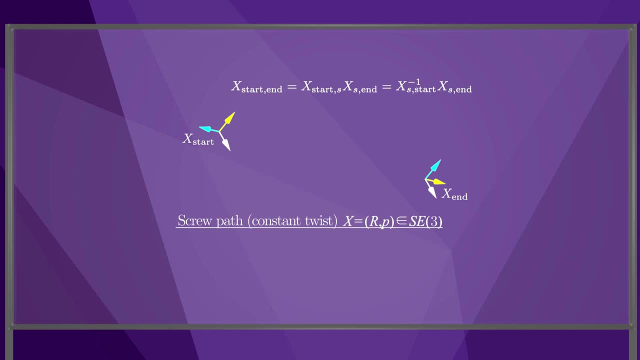 subscript cancellation rule. we find that X start inverse times, X end is the configuration of the end frame and the start frame. The log of this is the little SE representation of the twist expressed in the start frame that takes the start frame to the end frame in unit time. So our formula for the path. 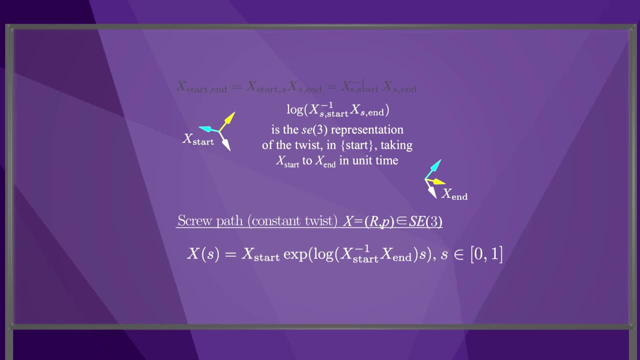 is X of S equals X start times the matrix exponential of S times the log of X start inverse times X end as S goes from 0 to 1.. The matrix exponential is multiplied on the right, since the twist is expressed in the start frame, not the 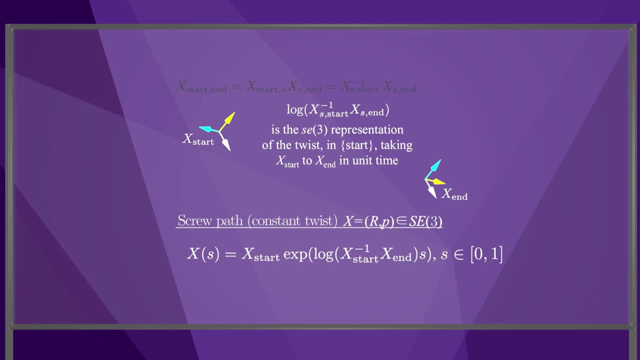 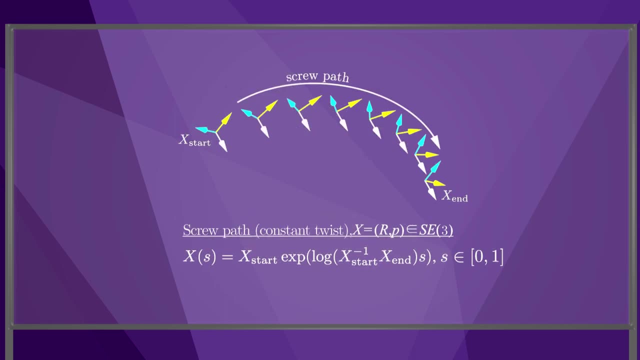 space frame. The path parameter S determines how far we follow the twist that takes the start frame to the end frame. The final screw path can be visualized as shown here. This is a straight line path in the sense that the twist is constant throughout the motion. Another type of path between X, start and 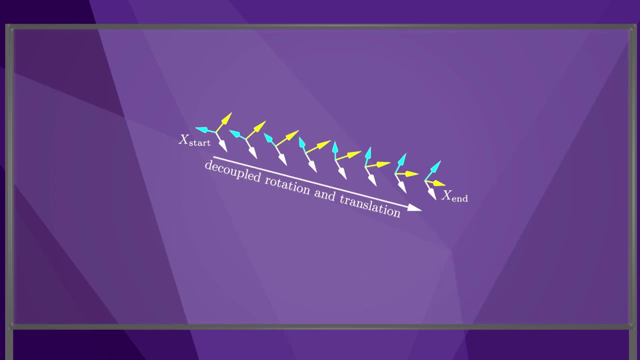 X end is one that decouples the rotation and translation. The origin of the frame follows a straight line and the rotation is about an axis fixed in the frame. For this type of path, the position coordinates P follow a straight line path for coordinates as discussed.